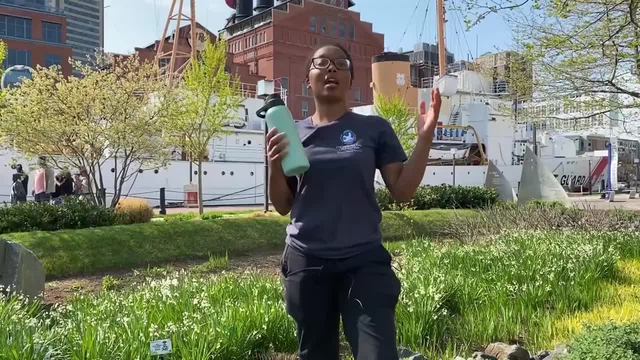 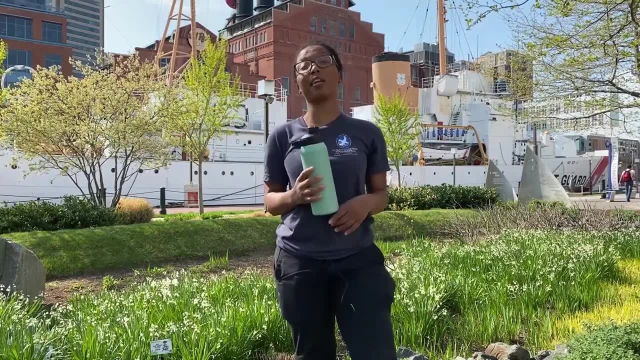 or they can be soft surfaces like soil or even grass. Now I want you to make a hypothesis about which surfaces will absorb water and which ones will not. Now, remember, a hypothesis is an educated guess about how changing one thing, your independent variable, will affect another. 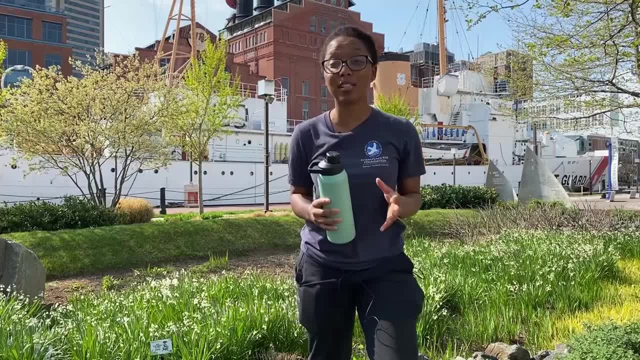 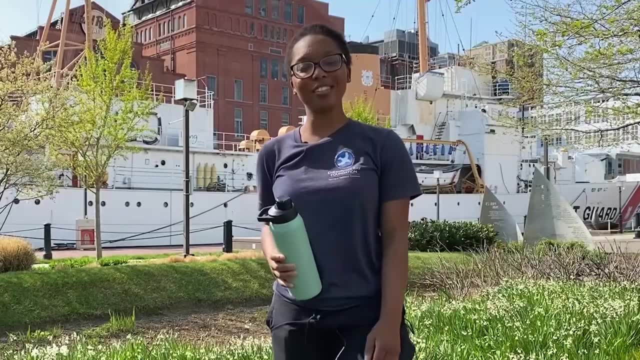 your dependent variable. I want you to go ahead and base your hypothesis on past observations. during a rainstorm, It is best if you can use an if-then statement. Not sure how to get started? Let me introduce you to a few friends who can help us out. My name is Elisha Carcomo and I'm 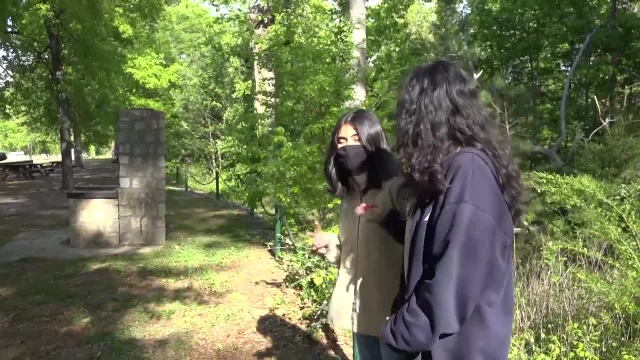 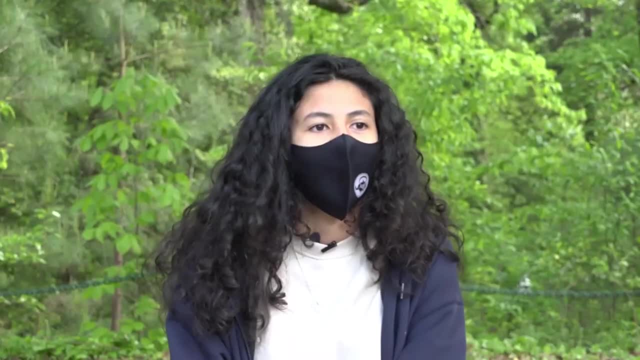 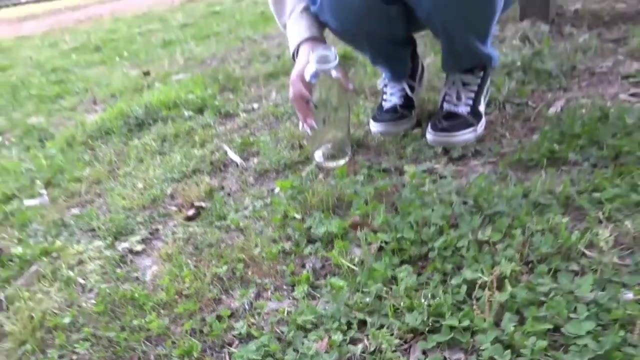 18 years old. My name is Amaya Carcomo. We did an experiment to see if we could find a way to see how fast or how far water can run on different surfaces. We did an experiment on pouring water on three different types of land: on concrete, a grassy area and a bushy area. They all 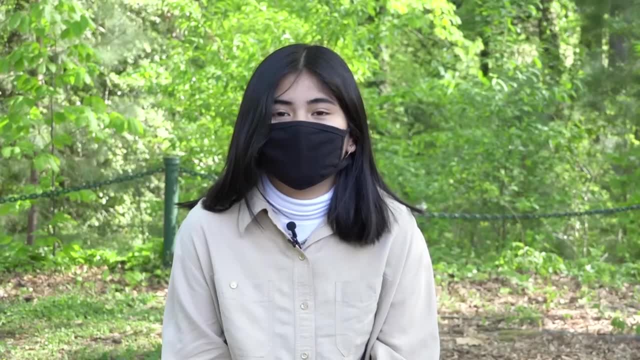 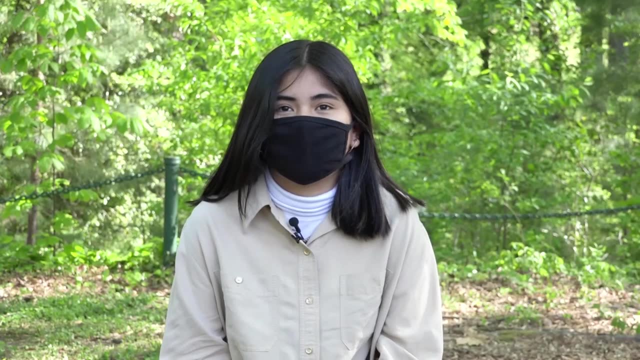 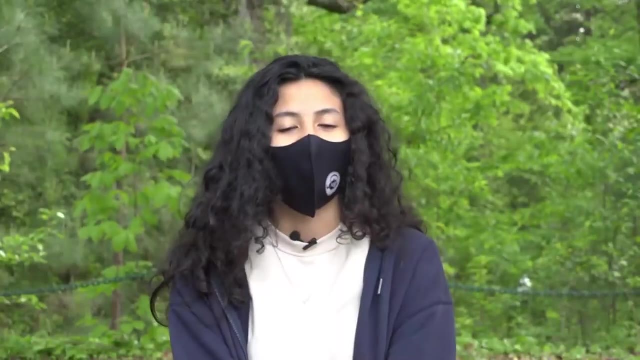 had a downward slope to help the water go down. Every time we poured the water we took a measurement to see how far it would get for each one. Our hypothesis was that on the water on concrete would go faster or further Because it's a solid. I was shocked to see that, even though we poured the same amount of water, 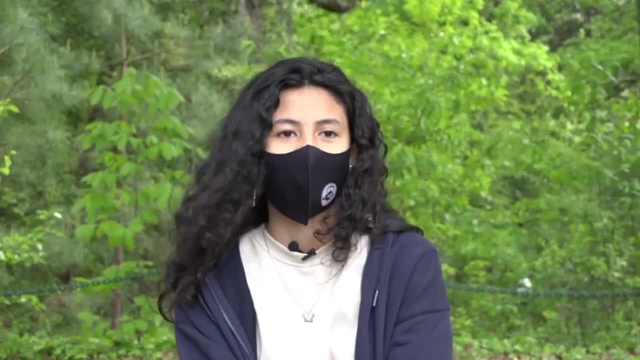 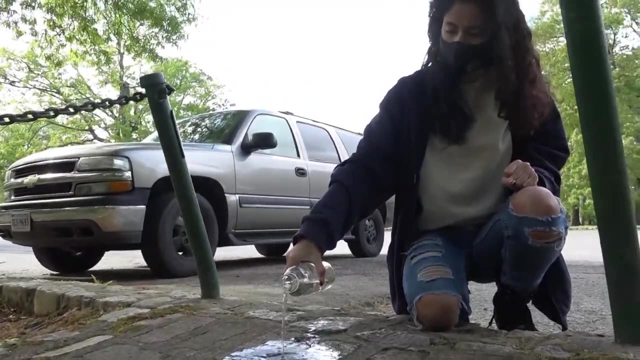 in the three different spots the outcome was very, very different. When I poured the water on the concrete, it's actually spread pretty quickly, pretty fast. It didn't show any in the tensions of stopping and it definitely if there was any kind of oil substance on there, it would. 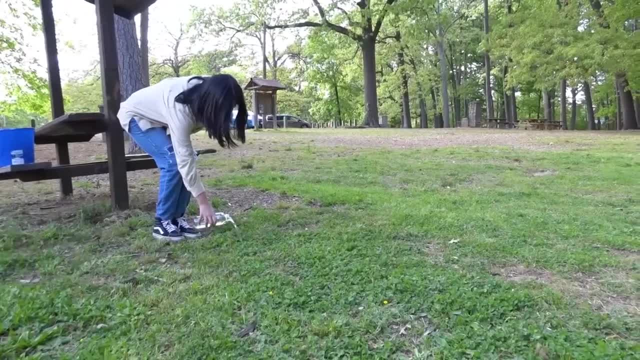 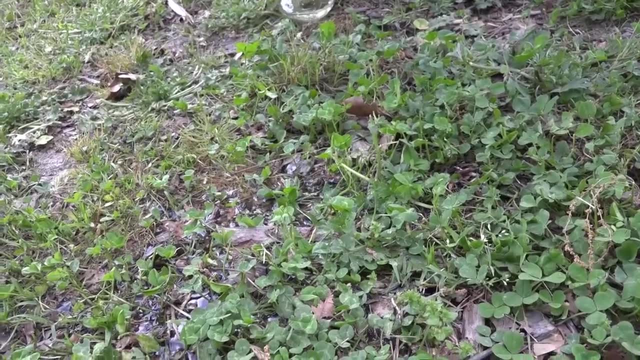 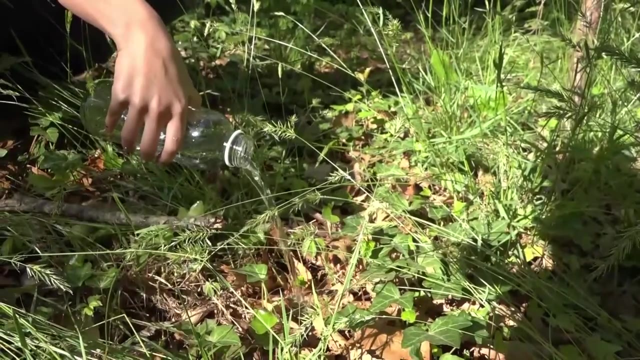 spread downward pretty fast. On the grassy area when we first poured the water it did take a while for it to spread out, but then it did spread out, just not as much as it did on the concrete. When I pour the water in the bushy area it didn't spread as much as the grassy area or the 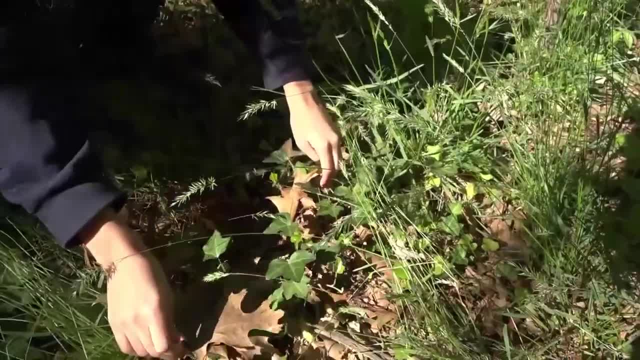 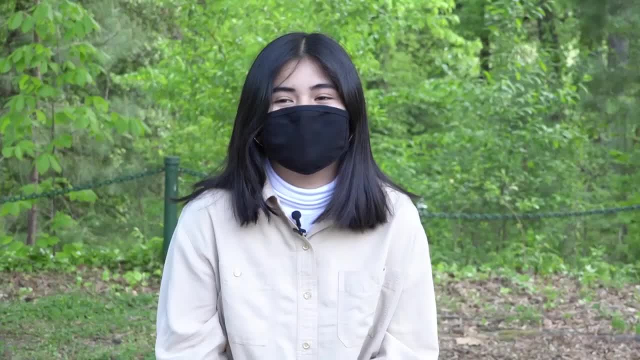 concrete area actually stayed in the same spot. All the leaves that were there, and also the grass and any other plant that was there, absorbed it pretty fast, so it didn't give it a chance to spread out. Parking lots and sidewalks are more likely to let the water go down easily, which will cause